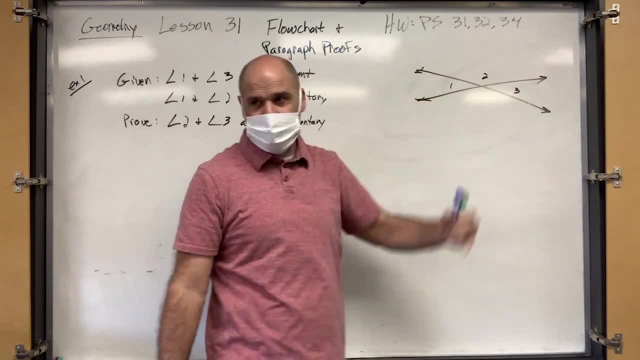 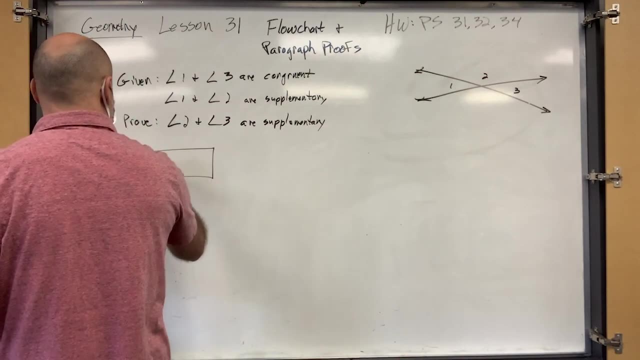 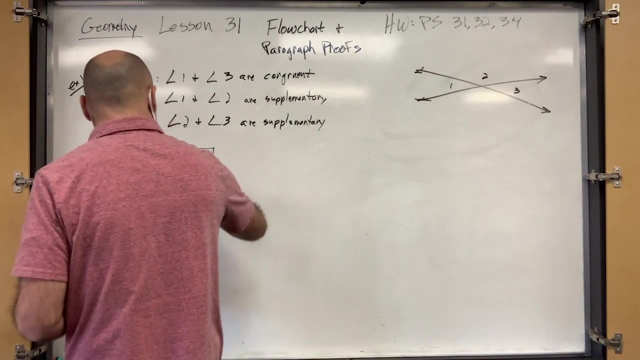 So I'm going to prove that angle three and angle two are supplementary. Okay, so here's the first part of my flow chart. Angle one and angle three are congruent, Or let's just say angle one congruent to angle three. 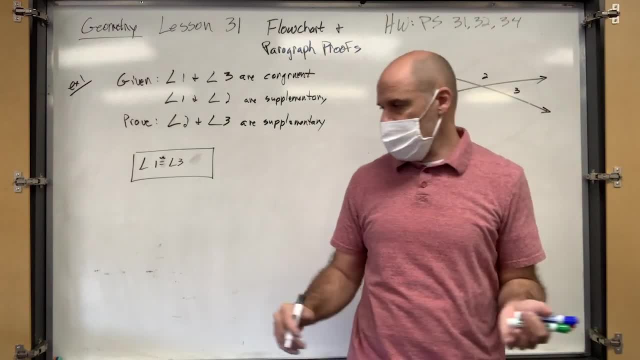 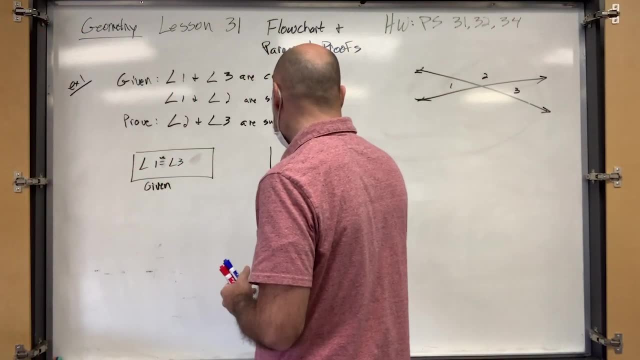 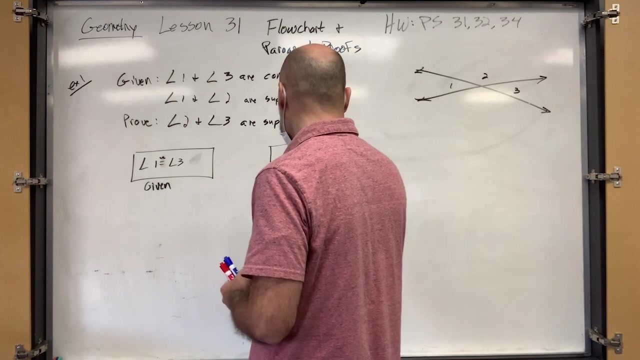 Why can we say that It's given? It's given, So I'm just going to write given underneath here. The other thing that's given is another part of my flow chart. Angle one and angle two are supplementary. Why? Because it's given. 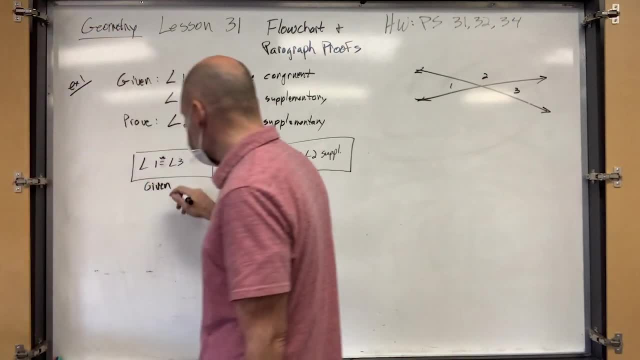 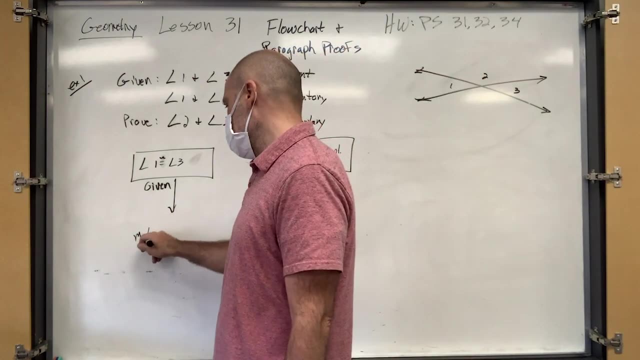 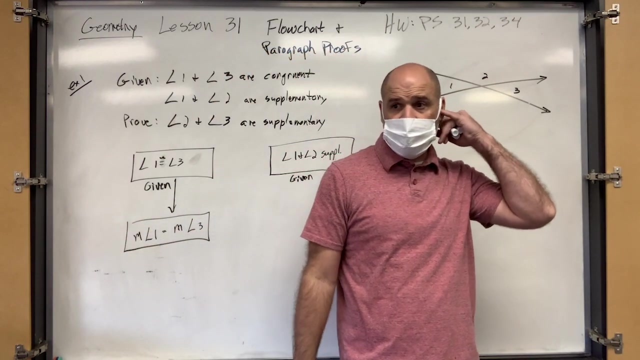 Okay, so here's what I can say. Okay, so here's what I can say. Here's what flows from this statement: The measure of angle one equals the measure of angle three. Why can we say that? So the only thing we know so far is that angle one is congruent to angle three. 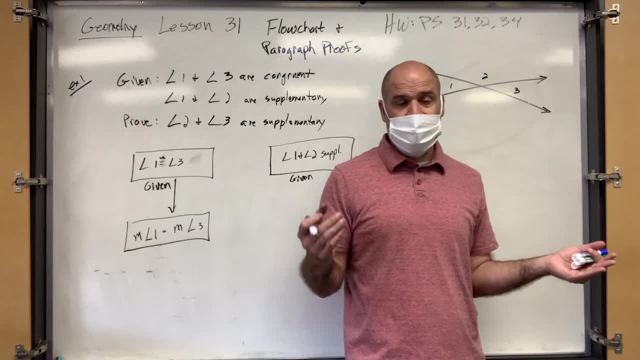 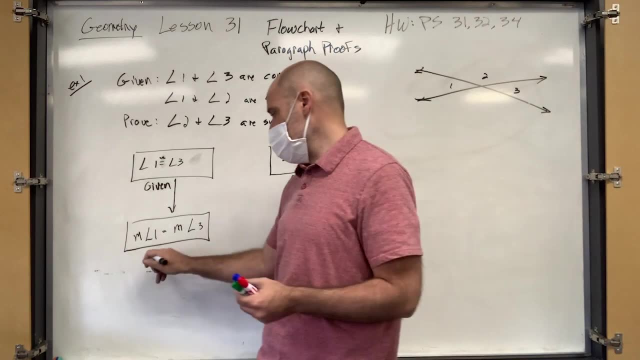 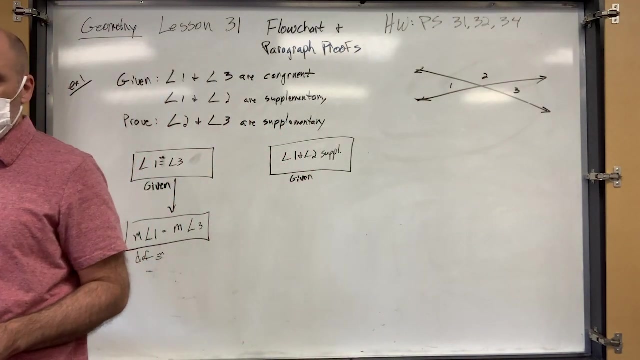 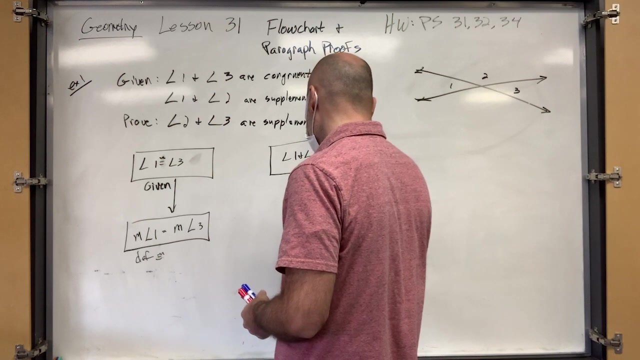 Then what gives us the right to say measure of angle one equals measure of angle three. Yeah, that's what congruent means. So definition of congruent Def. congruence. Meanwhile, I could say this: Measure of angle one plus measure of angle two equals 180. 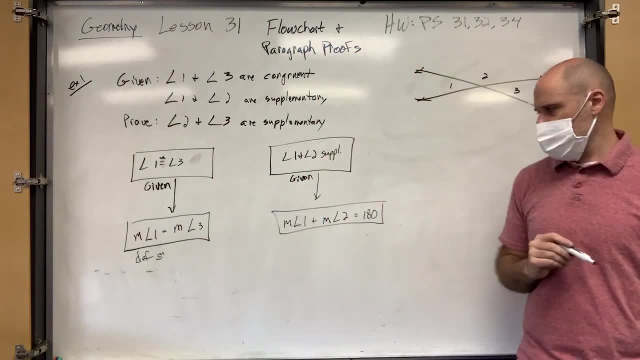 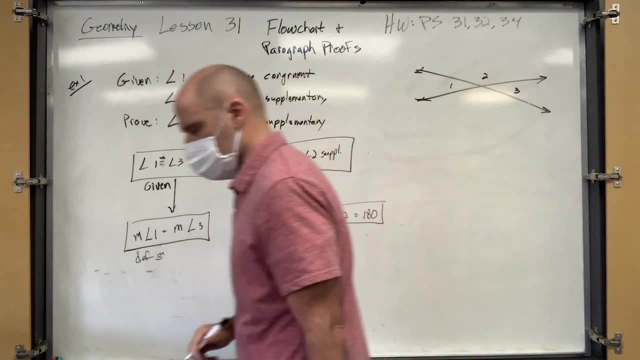 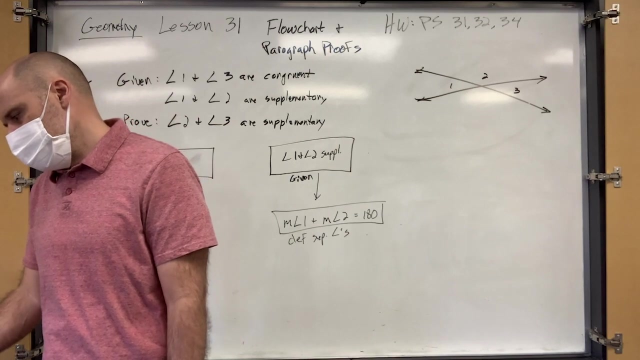 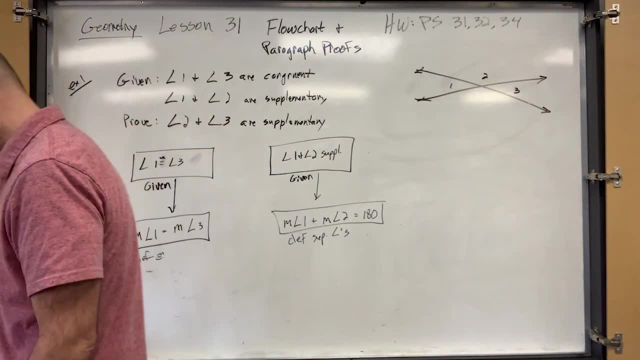 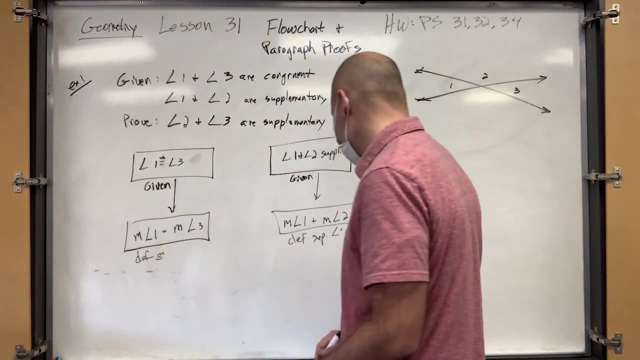 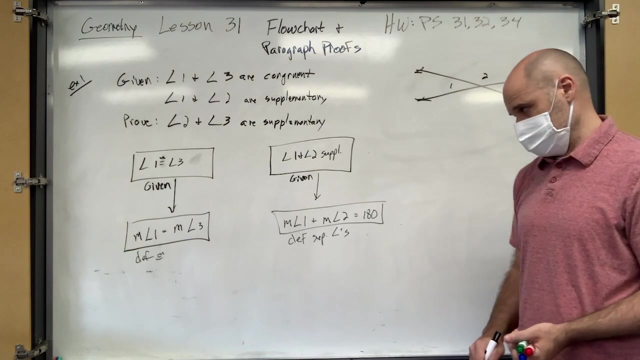 Left dy is lower Right dy. equaler Right dy. equaler Def На equal dY. equal dY. equal f equals one Right dy equal. Okay, So now I can say: here's what I'm going to do. 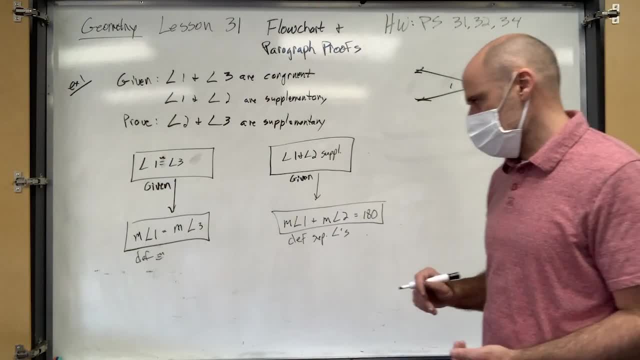 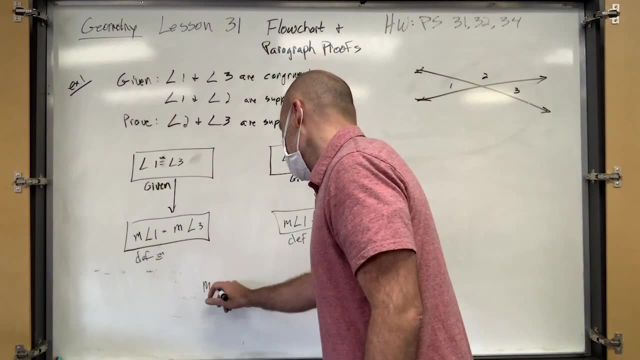 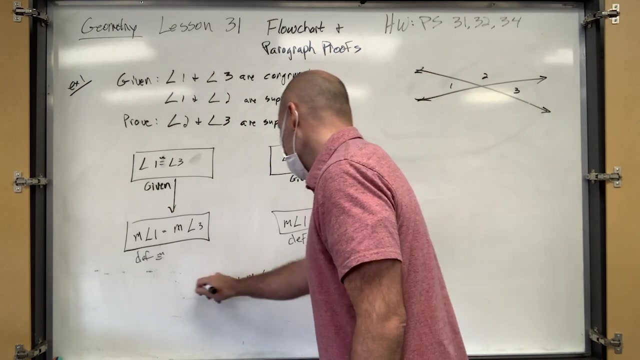 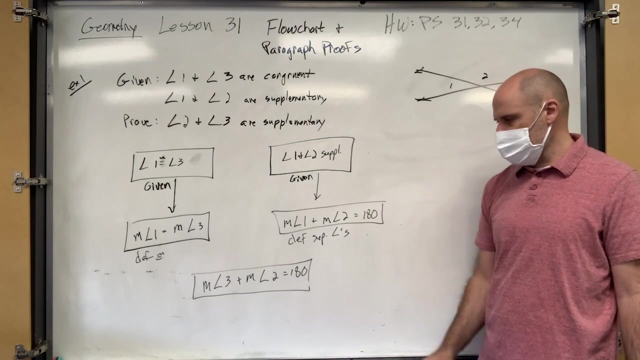 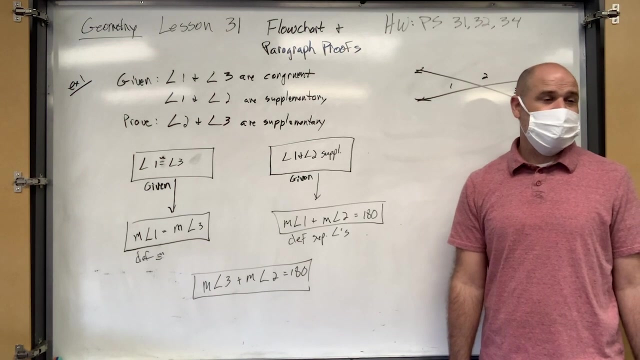 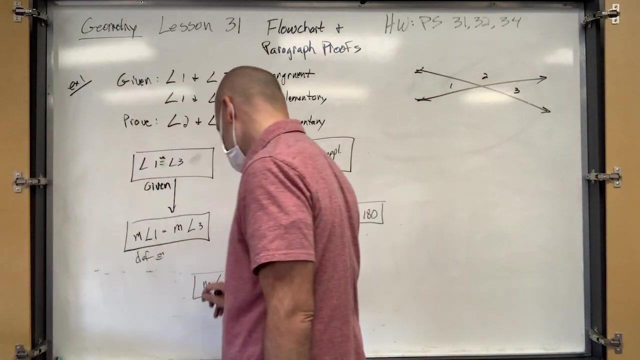 Yes, Yes, Yes, Yes, Yes. so now I can say: measure of angle 3 plus measure of angle 2 equals 180. why can I say that? what's the difference between here and here? yeah, it's been. what's another word for replaced, substituted, so this is substitution, property of equality. now these 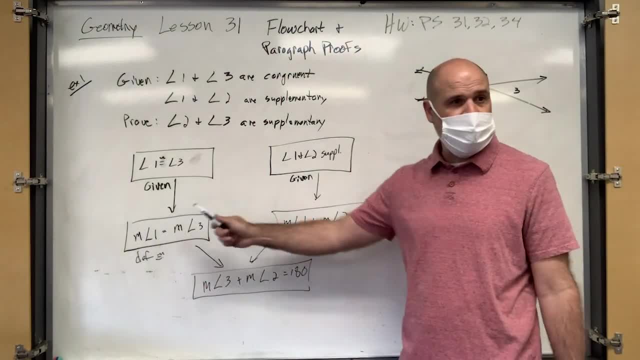 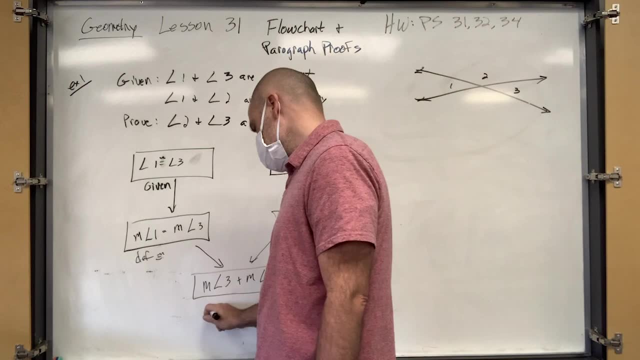 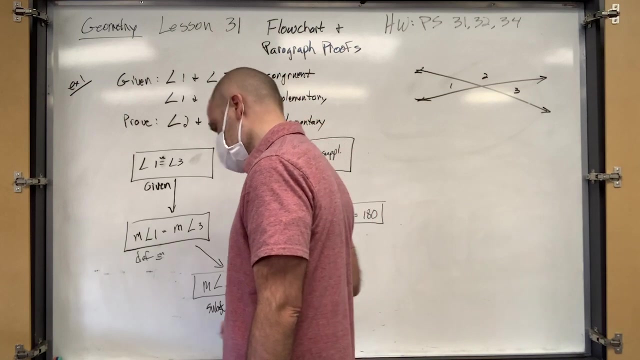 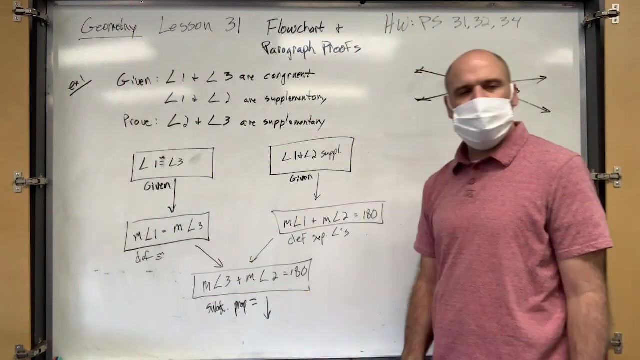 both coat from here. so I use both of this information to say that this statement, because I can substitute that in there. so this is the substitution. so stick prop equality. okay. so now what: I haven't proven anything yet. I haven't said what my last statement, which it: 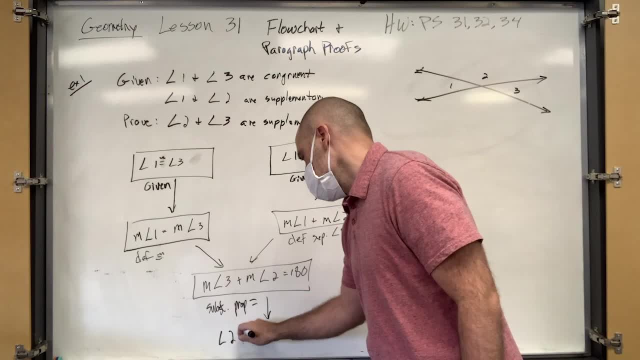 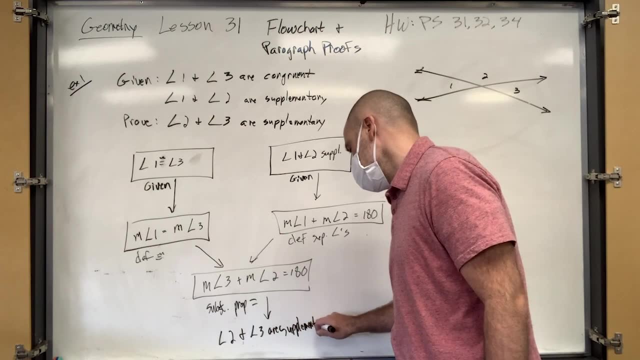 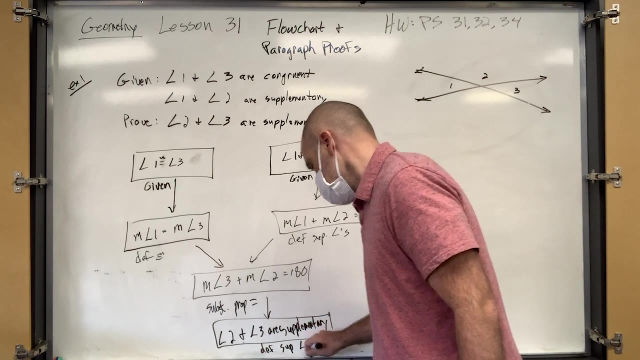 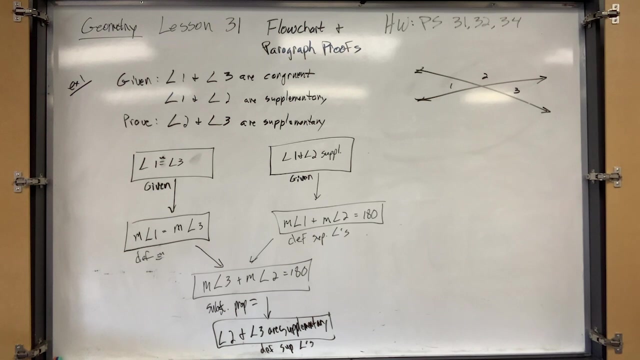 should be: angle 2 and angle 3 are supplementary. why can I say that? right back to the definition of supplementary depth sup angles, that's okay. so now what? I haven't proven anything yet. I haven't said what my last statement, which it should be: angle 2 and angle 3 are supplementary. why can I say that? right back to the definition. 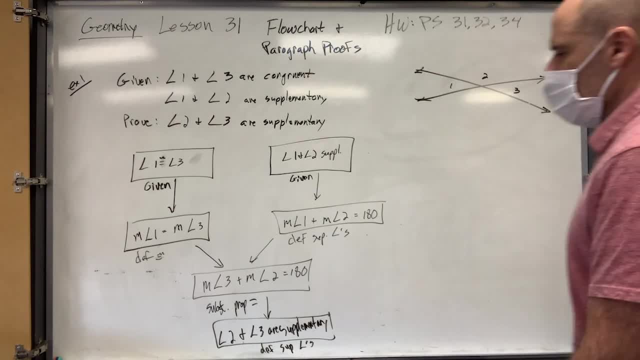 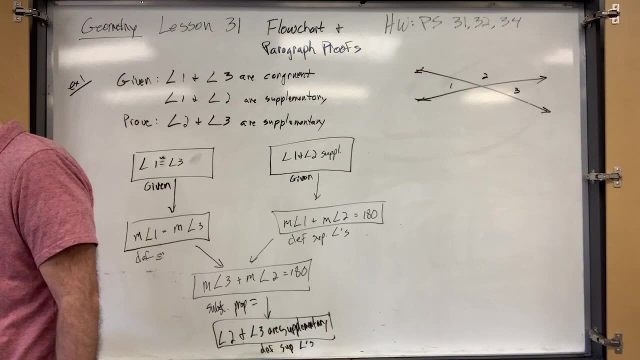 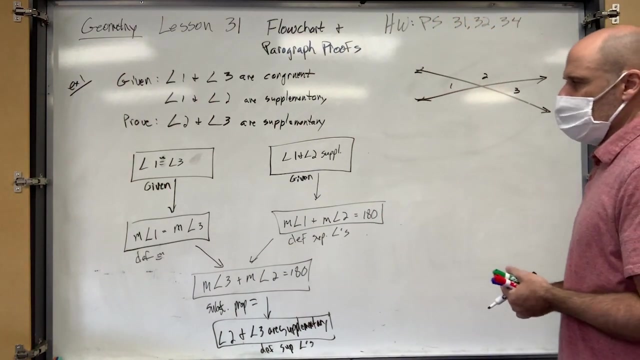 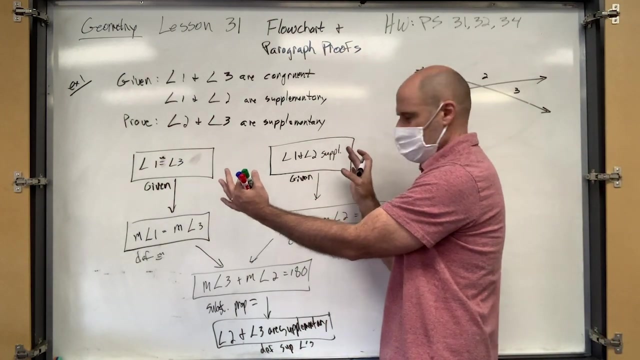 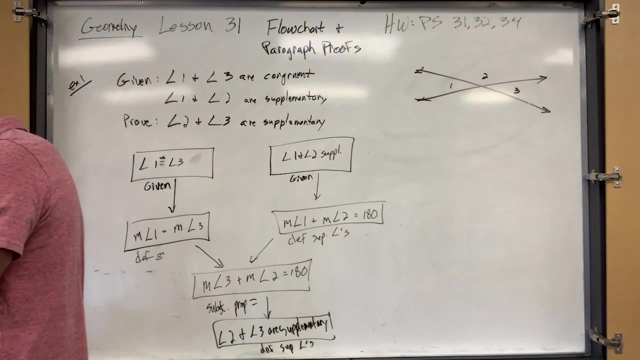 of supplementary depth sup angles. that's okay. so now what? I haven't proven anything yet I haven't said what. my last statement, which it should be angle 3 are supplementary. why can I say that? right back to the definition. okay, what I've proved. so this is the approach I took from candle formula. it's now appropriate to. 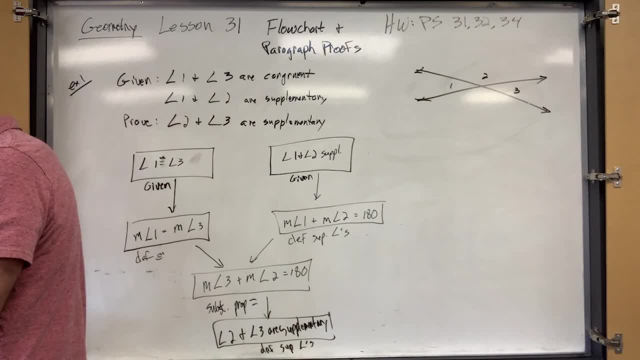 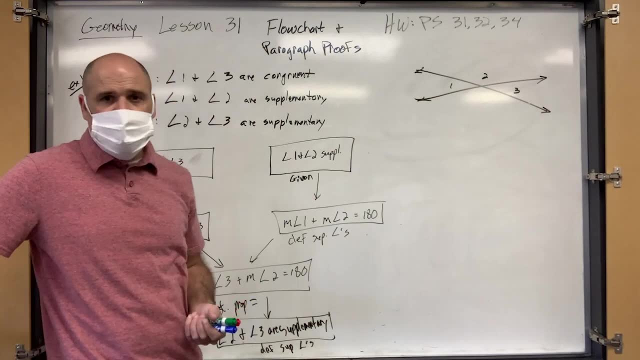 a specific disagreement, okay. so at the very end you decide it's better here than here, okay. and also, I went to a point where there were notes. if you didn't know, well, when you heard that, you knew that, you knew that, and if you not want to forget what that means, where you want to forget what that 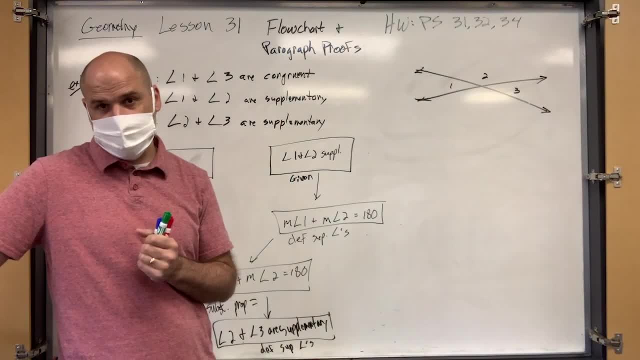 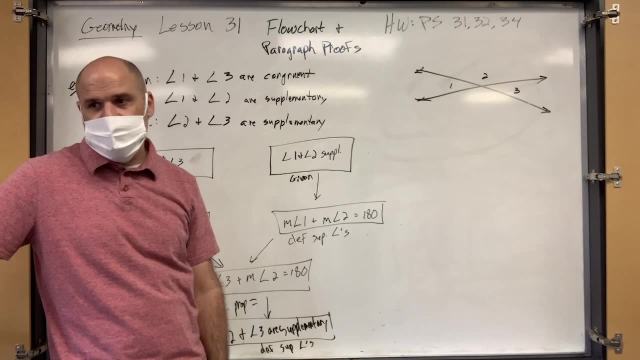 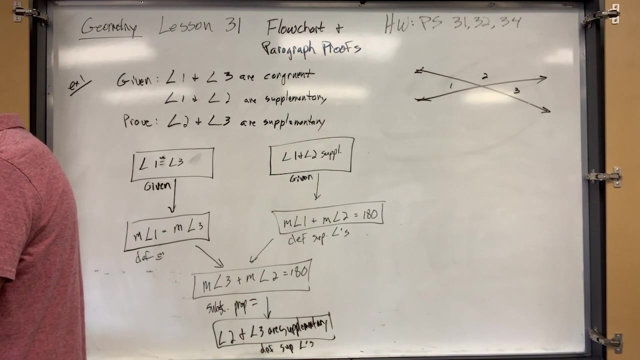 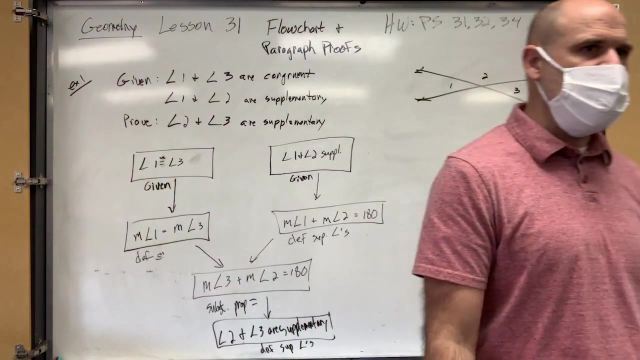 are two different types of people. okay, I am such a linear list type of person, maybe. yeah, just tell me what I need to do and I'll do it. just give me the list. yeah, okay, so a paragraph proof is very similar to this, but you're just using complete. 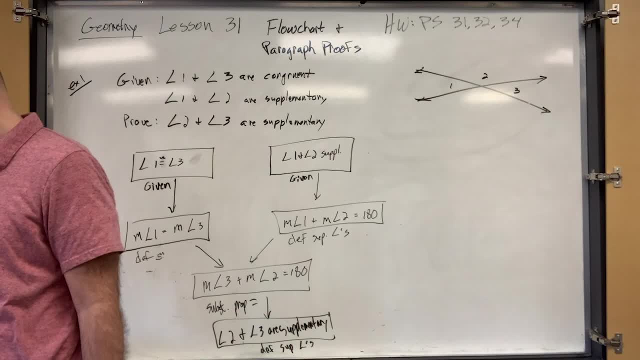 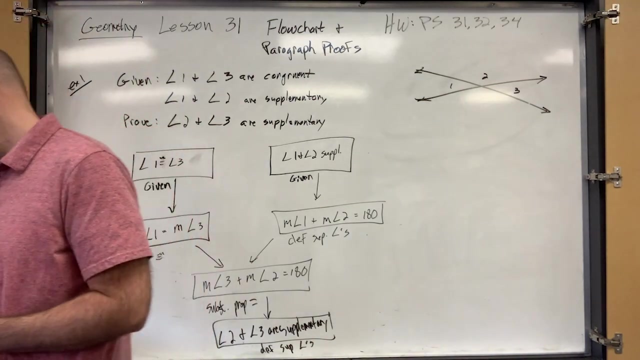 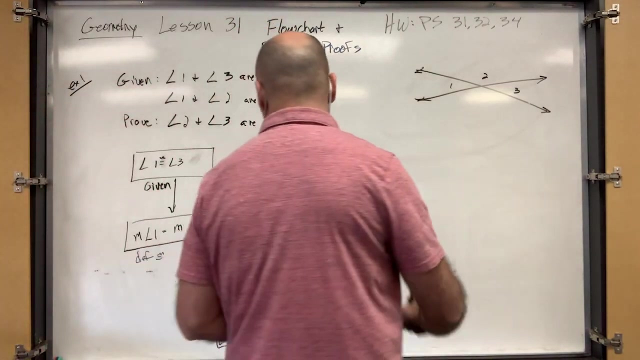 sentences and just explaining what you see right. so I could say. I could say something like this: angle one is congruent to angle three. so measure of angle one equals the measure of angle three. okay, by the definition of congruency I could just spell it all out. I could say: since: 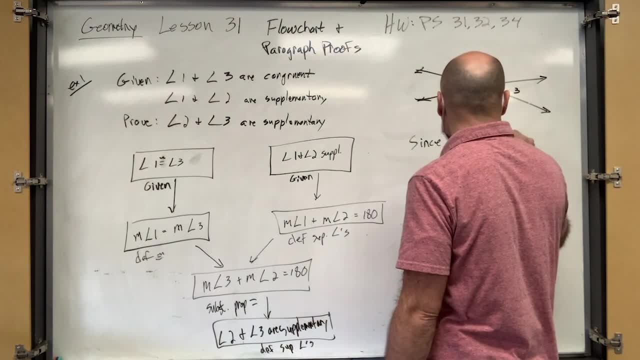 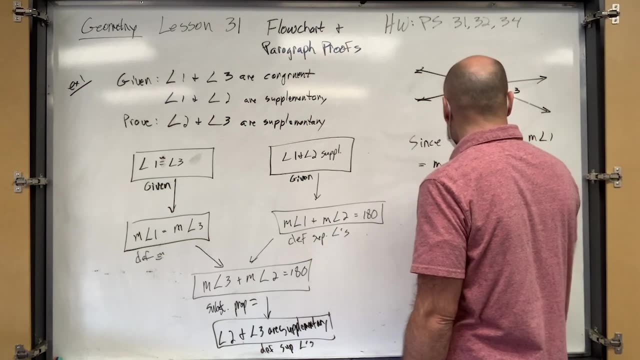 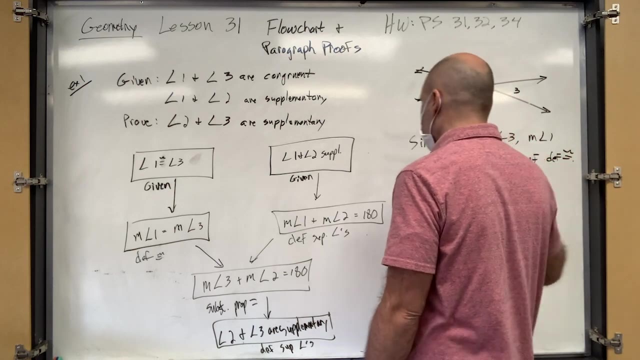 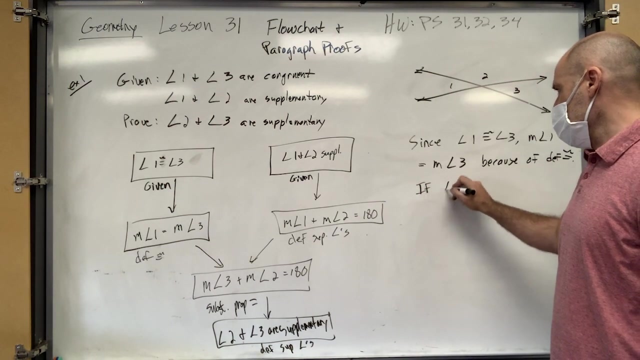 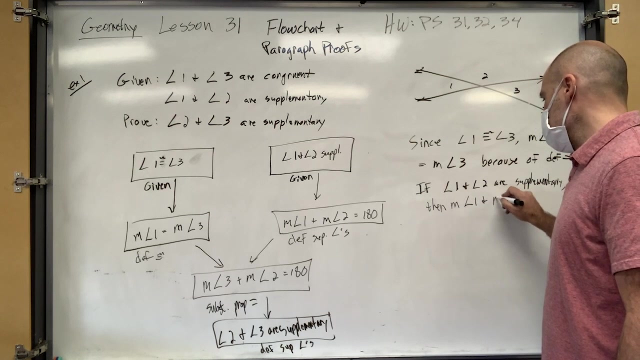 angle one is congruent to angle three. measure of angle one equals the measure of angle three because of the definition of congruency. okay, and then I can say, by the definition of congruency, if angle one and angle two are supplementary, then measure of angle one plus measure of angle two equals 180. 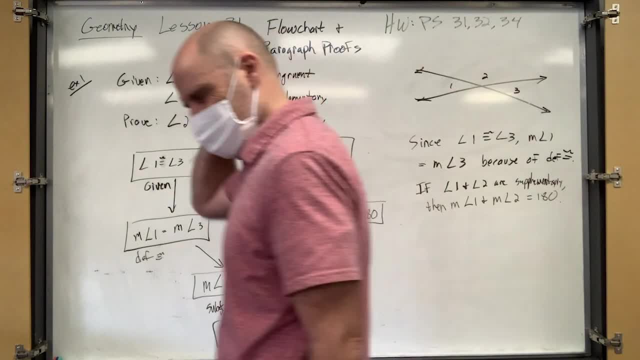 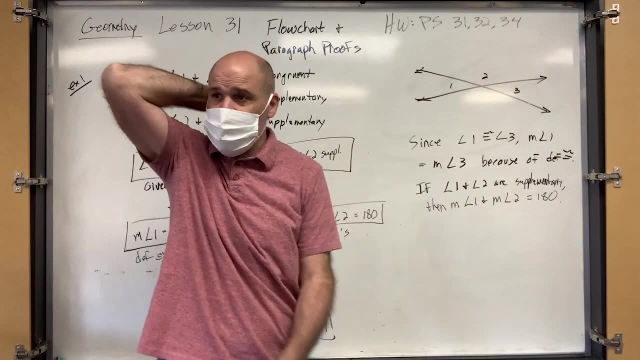 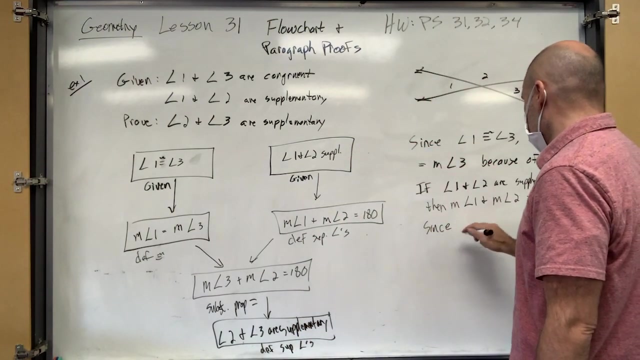 and then I could probably just say, yes, I don't even have to say why, because I just did. and, and since they're supplementary, I can say, yes, I don't have to say why, because I just did, and since they're, then they add up to 180, okay. and then I can say, since measure of angle 1 equals, 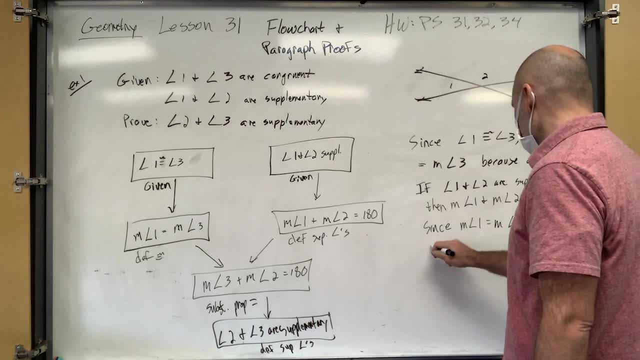 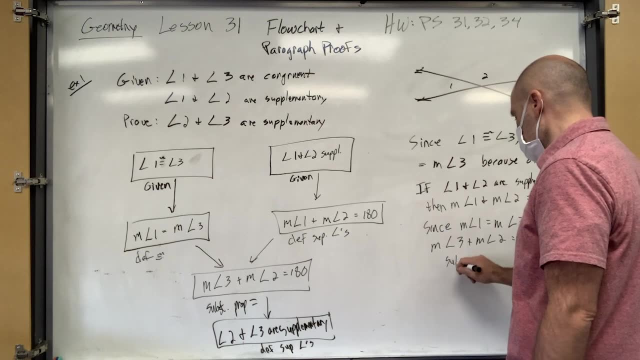 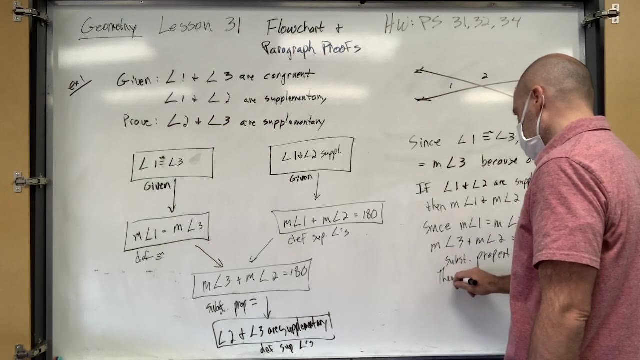 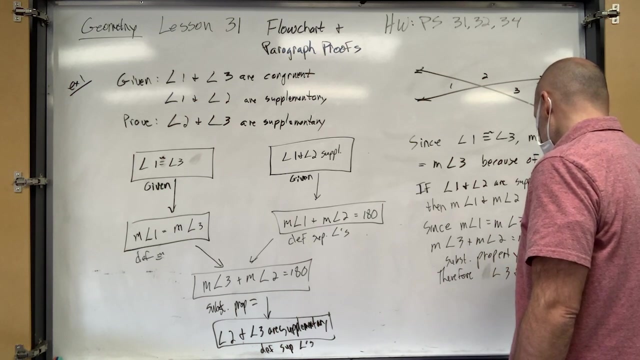 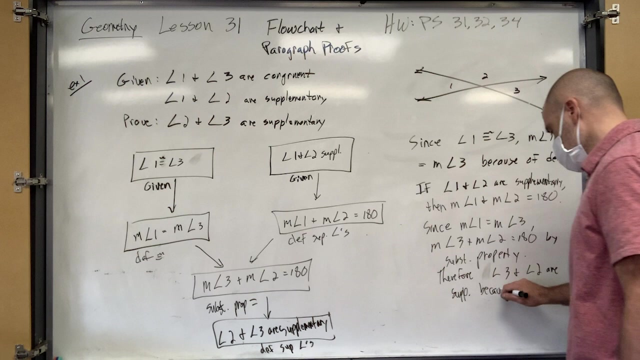 measure of angle 3. measure of angle 3 plus measure of angle 2 equals 180 by the substitution property. therefore, measure of angle 3 for angle 3 and angle 2 are supplementary because of the definition of supplementary. so this is kind of a pain in the butt. 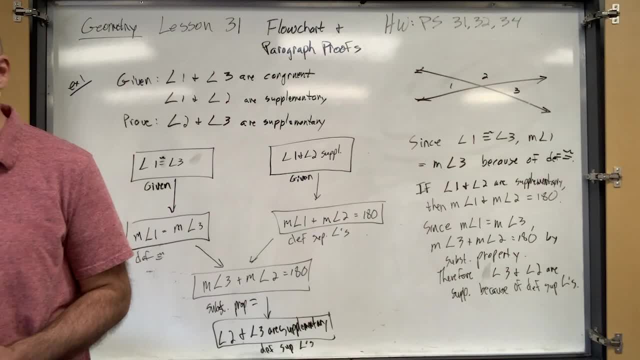 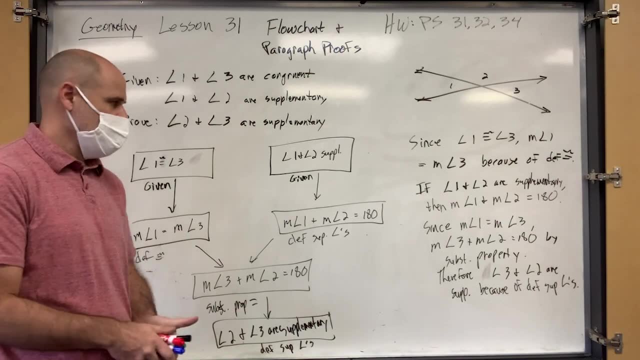 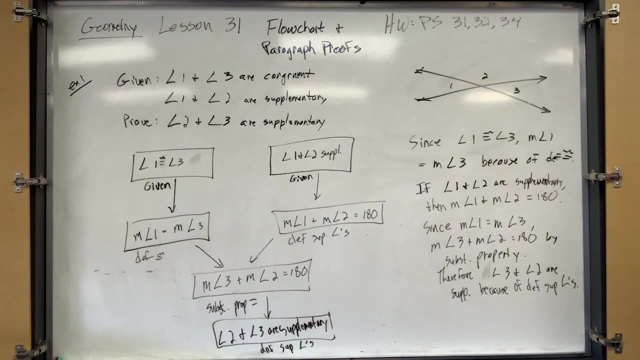 I don't like writing reports. I don't like writing papers. this is what a paragraph proof seems like to me, just explaining everything in detail. okay now, um, if you go into law- we already talked about how geometry is a great preparation for law, because, yeah, you have to. your goal is to make 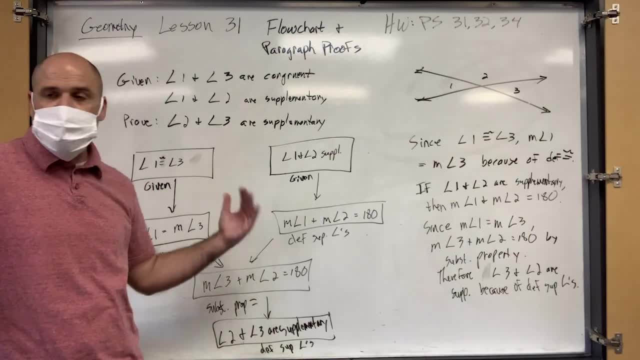 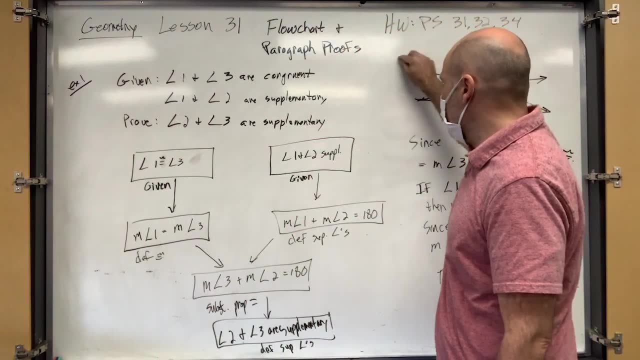 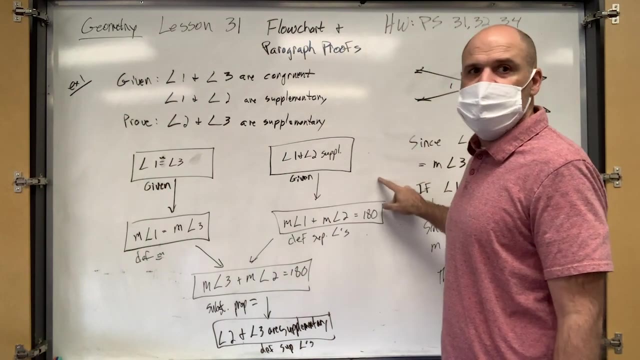 everyone in the room feel stupid. okay, so you can be as detailed as you want. you can have a flow chart like: here's the here's Jack. Jack finds knife. Jack gets fingerprints on knife. Sally is dead. no one else is in the room. a little flow chart proof: in the courtroom. you feel stupid. 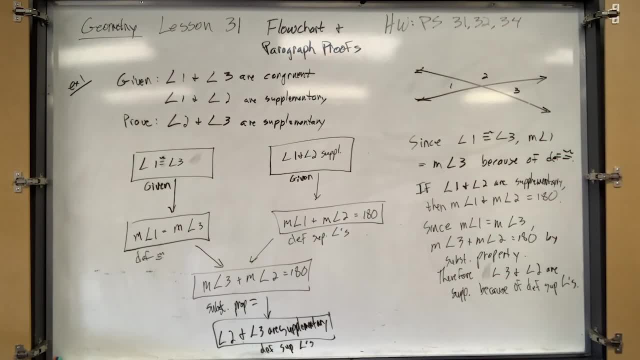 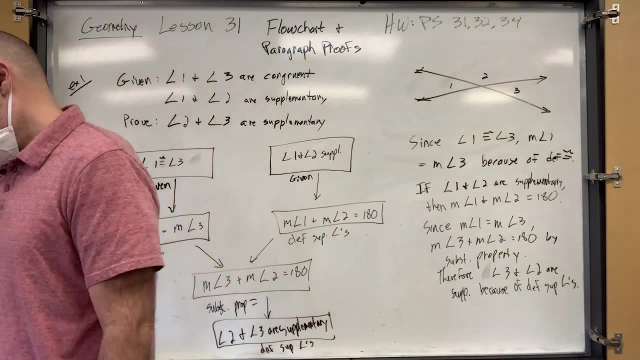 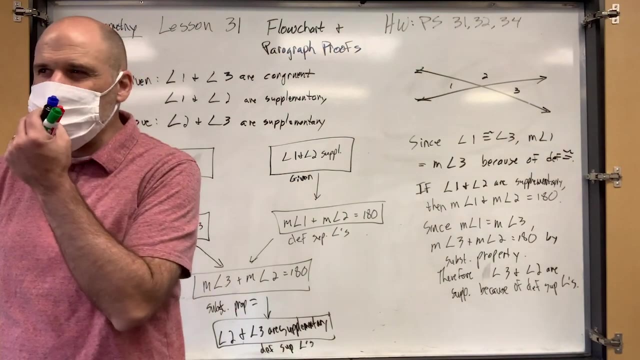 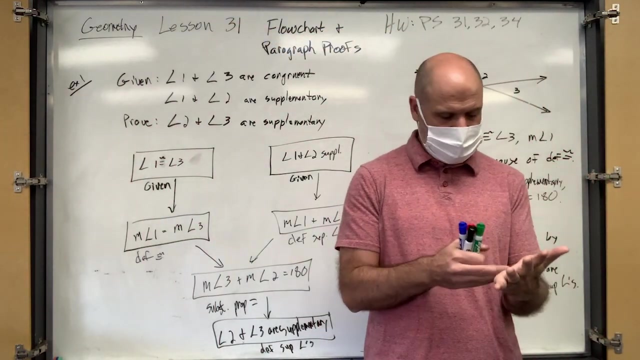 but it's undeniable that Jack is a jerk because he kills. he killed Sally, okay, okay, so these are just different types of proofs. um, you, you might be tested on it like a paragraph proof, but um, if you are, we're going to go over it in detail before, so don't. 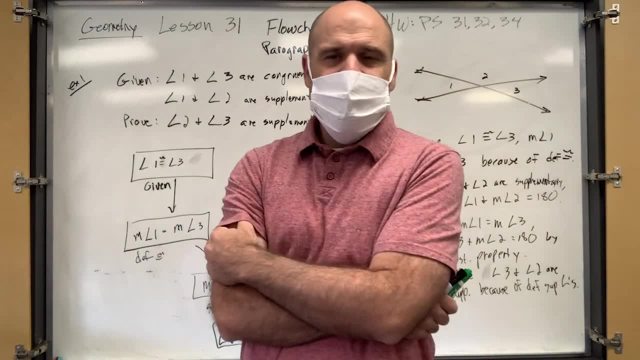 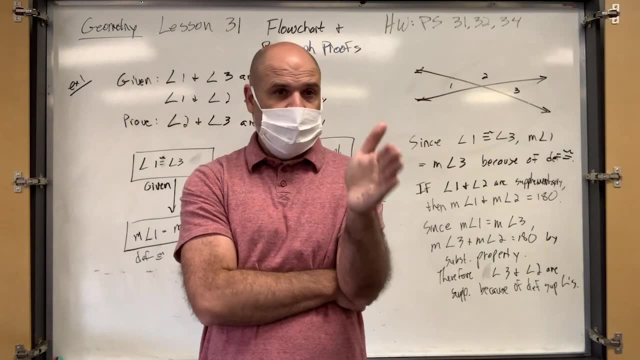 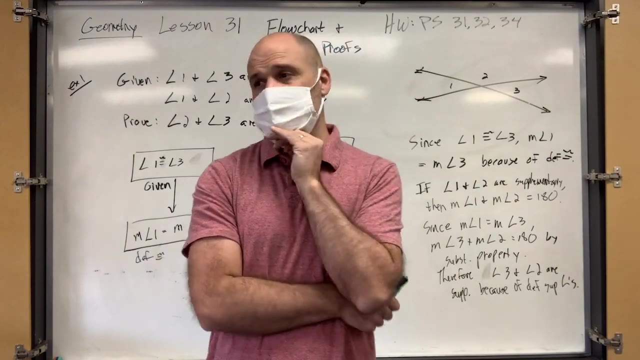 don't stress too much about it, but either way, you have to begin the process of walking people through an argument step by step, with a justification of each step. okay, whether that's with a flow chart or in a paragraph, and there's lots of senses, ifs and 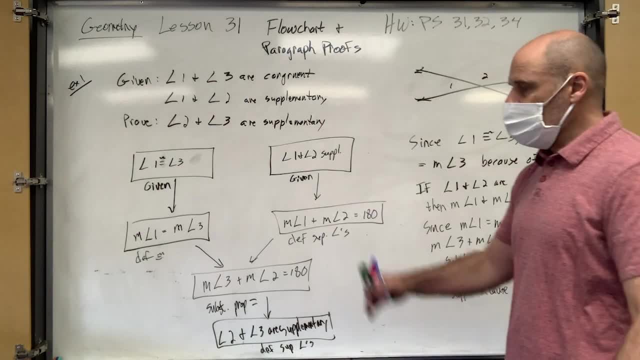 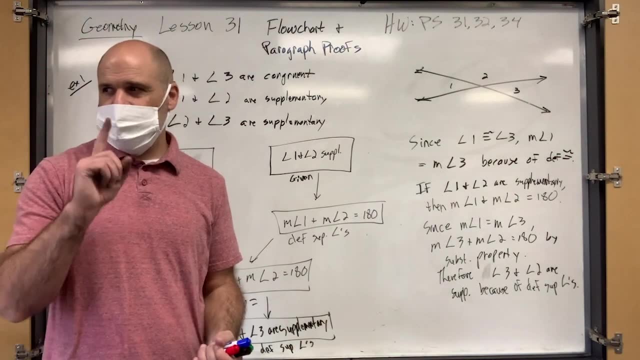 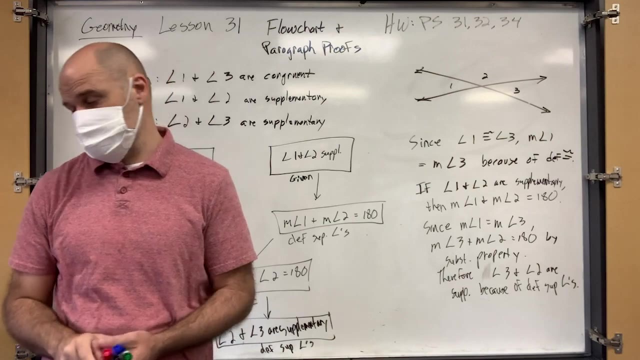 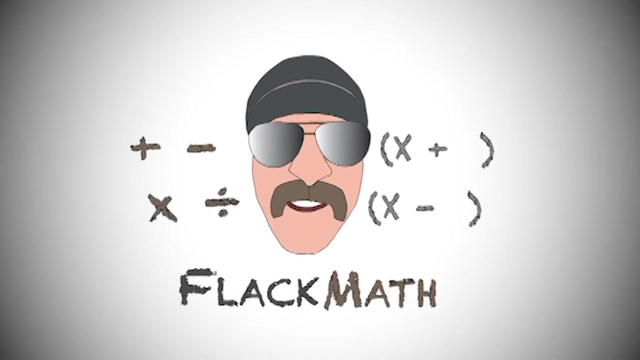 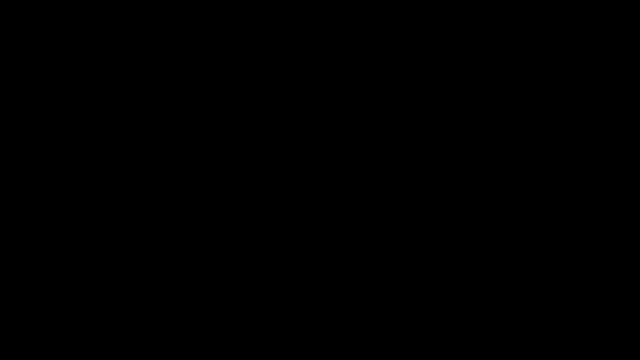 because in a paragraph proof or a two-column proof. either way, either one of those options works. okay, just be as duh as you can. okay, explain everything over. explain, all right. so I'm going to move on to To the next lesson. Thank you.